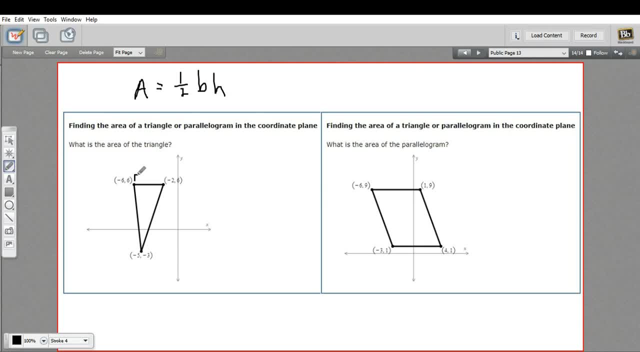 So for this particular triangle here we could make this side the base and we could know the length of the base just by subtracting the x-coordinates. We would get a distance of four. here, Negative two to negative six is a distance of four. So base is four. 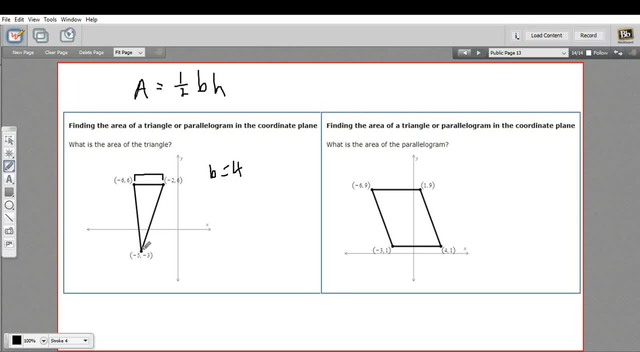 What about the height? Well, the height of a triangle, you start from the vertex opposite the base and you drop a perpendicular line, And we don't have a measurement for that. but the length of this line is the length of the base. The length of this line is the difference between the y-coordinates. 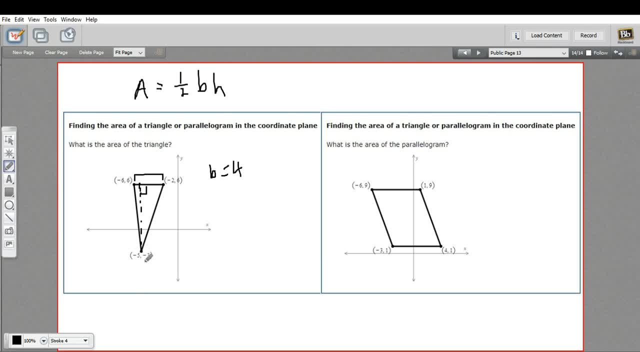 on the base and the y-coordinate here at the vertex. So our y-coordinate here is negative three. Our y-coordinate here is positive six. So that's a distance of nine. So our height equals nine. So now we can go ahead and plug everything into the formula. The area is one half. 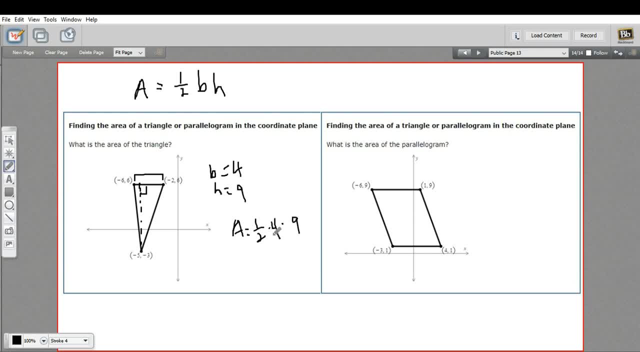 the base times the height, And one half of four is two times nine, So our area equals 18, and, and we just say square units here. So for a parallelogram it's pretty similar. The formula, though, is: the area equals the base times the height. So we can say: this is our base, and we'll 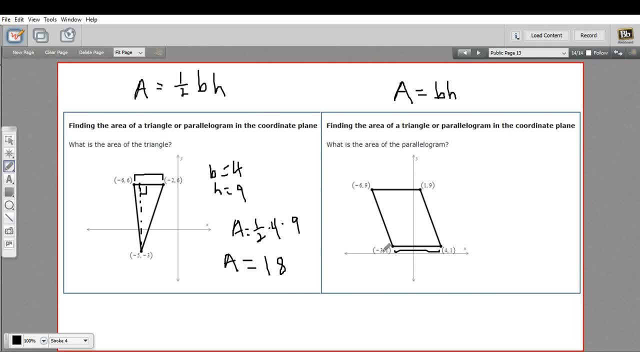 find the length of that by looking at the difference between the x-coordinates. So we have negative three up to four, That's a distance of seven, So that side is seven. And then in a parallelogram, we need a height, So we do the same thing. We need a height, So we do the same thing. 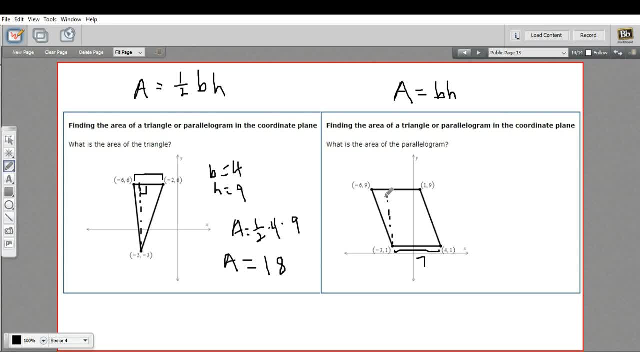 We take a perpendicular from one vertex to the opposite side And again this distance is going to be the difference in the y-coordinates. So we're going from one up to nine, That's eight. So our area here is just going to be the base times, the height, or 56 square units. So that's a little bit of weight.